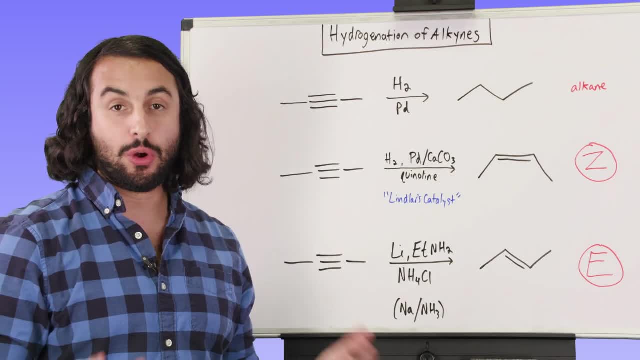 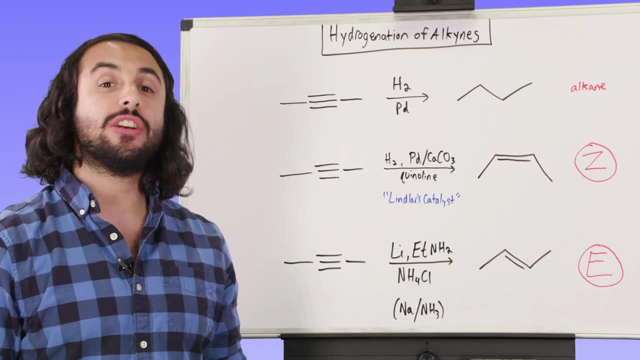 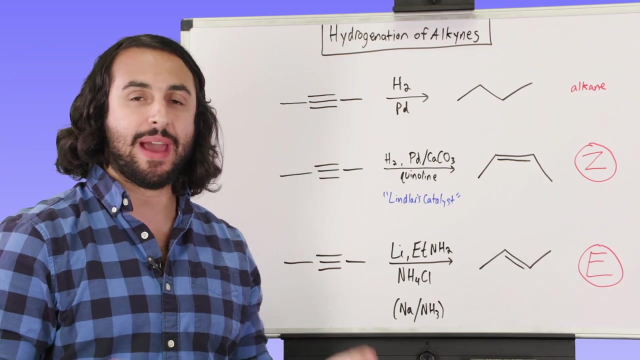 alkene and not go all the way to the alkene, And so there's a couple ways to do this. The first one looks like this: this is a situation, right? this is called Lindler's catalyst, and so what it is is it's hydrogen and it's some. it's always. it's a metal, it's. 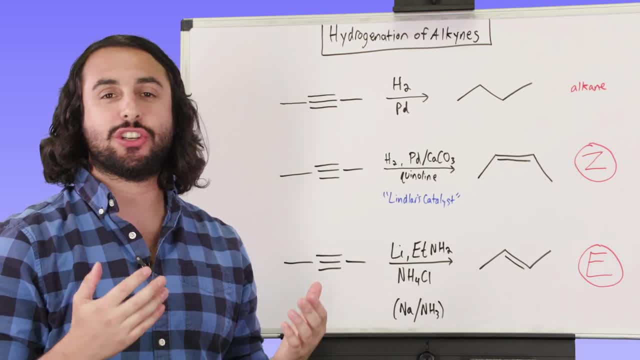 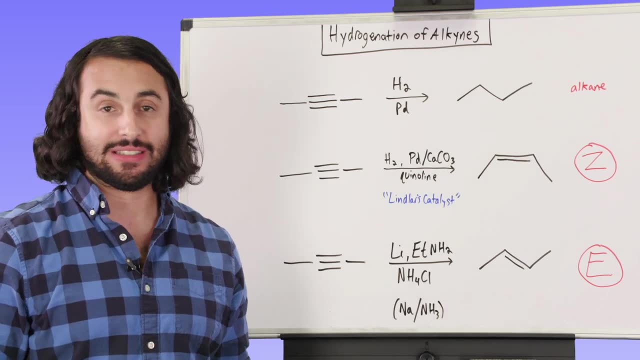 palladium, but it's been poisoned, and so what happens is that actually limits its ability to hydrogenate. it is only able to hydrogenate alkynes and not alkenes, And so it's going to be able to interact with this alkene and produce an alkene, but 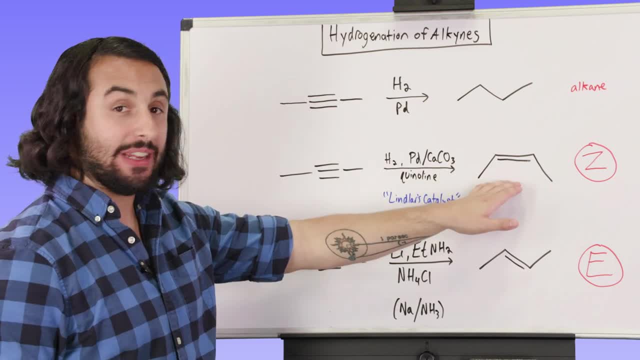 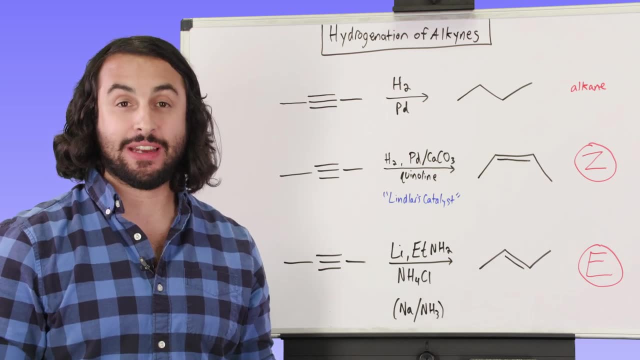 it is specifically going to produce the Z-alkene, right? so remember, when we have an alkene, we can have two different kinds of stereochemistry. we could have an E or a Z-alkene and, if you remember my tutorial, 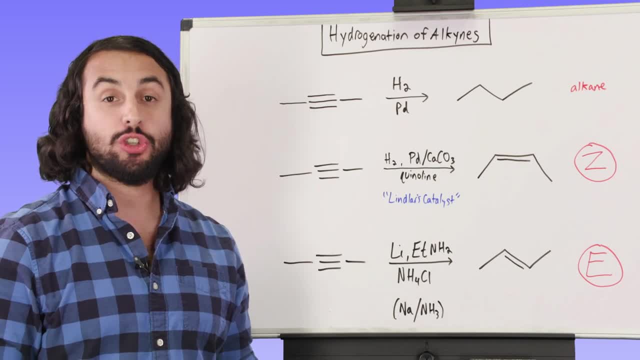 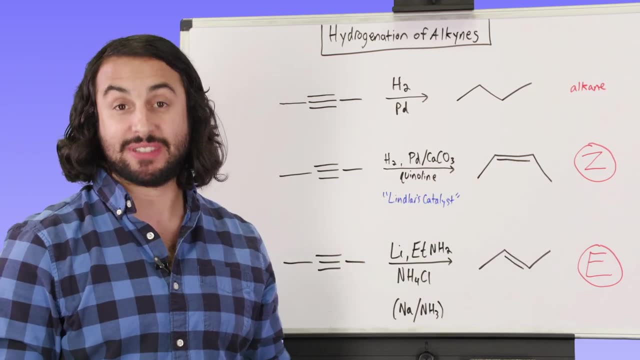 On this. we talked about how to use the Kahn-Ingold prelog convention to assess whether an alkene is E or Z, and so in this case it's Z because, if you remember, Z-same-zide right. 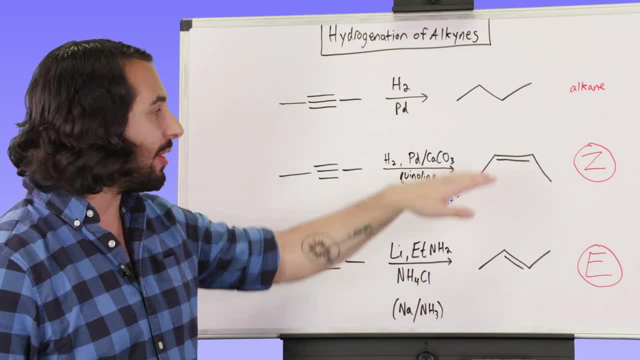 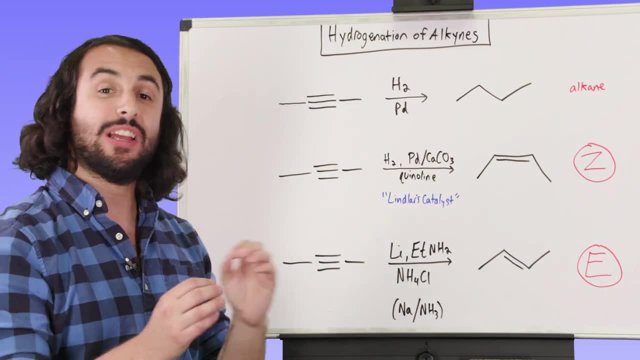 So these groups are on the same side of the plane containing the double bond. so this is a Z-alkene, and so when we see these conditions now there are a few variations. you may see it written a few different ways. often times you will just see the words. Lindler's catalyst. 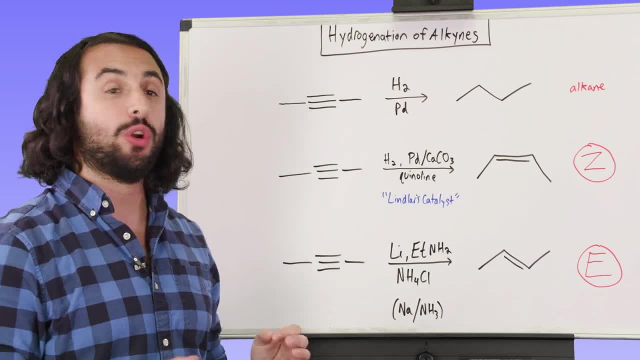 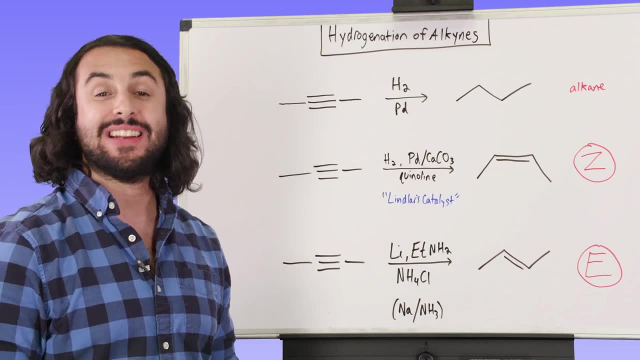 or simply Lindler, And so what this is telling us is that this is a Z-alkene. What this is telling us is: we know we're going from the alkene to the Z-alkene, okay, so that is one thing that we could do very deliberately in a synthetic pathway, if we 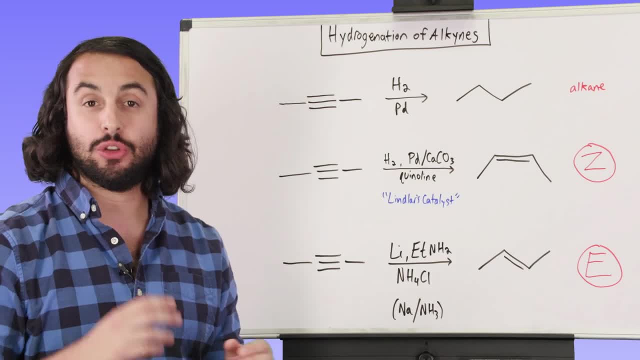 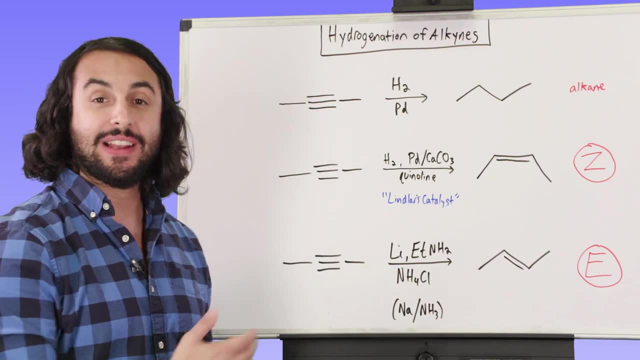 have an alkene and we want to get a Z-alkene to then do some other chemistry. Now, obviously, if we have a way to get the Z-alkene, we want to have a way to get the E-alkene as well, depending on what we're trying to do in our synthetic pathway. 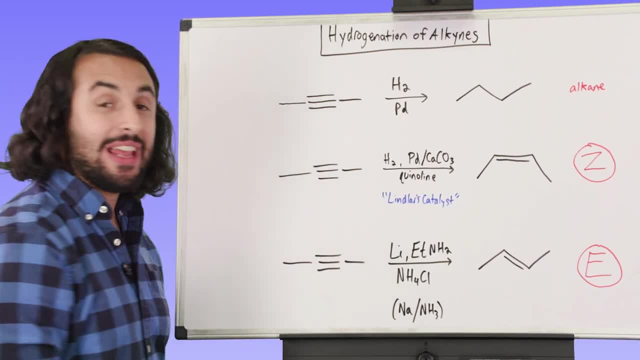 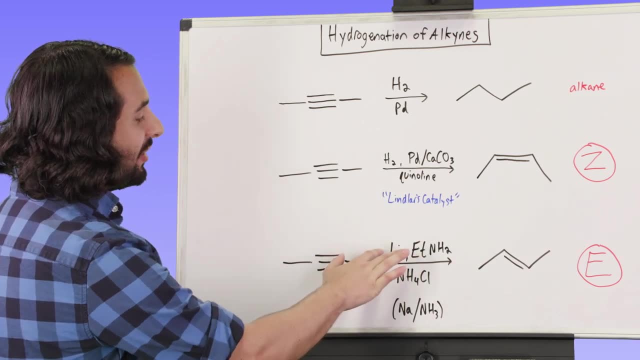 And so there's another way, and let's start with that same alkene one more time, and what we're seeing is that if we have this situation, we could see it like this with lithium and ethylamine and ammonium chloride. an alternate way that you will commonly see is sodium and 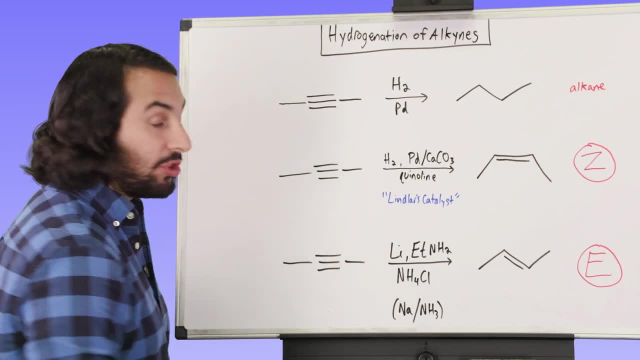 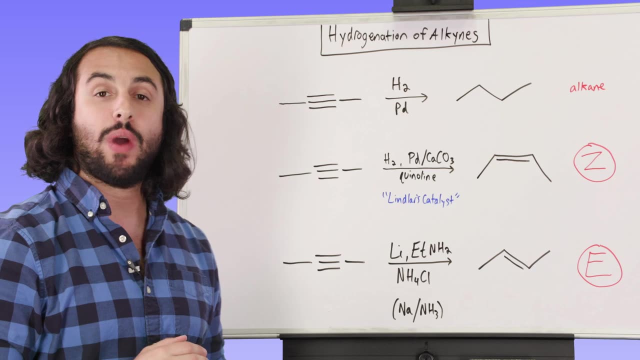 ammonia. so really, the key here is one of these metals, lithium or sodium, one of those alkali metals that is going to do this chemistry. it is going to, again, in a limited way. it's not going to be able to hydrogenate the alkene, so it is going to stop at the alkene functional. 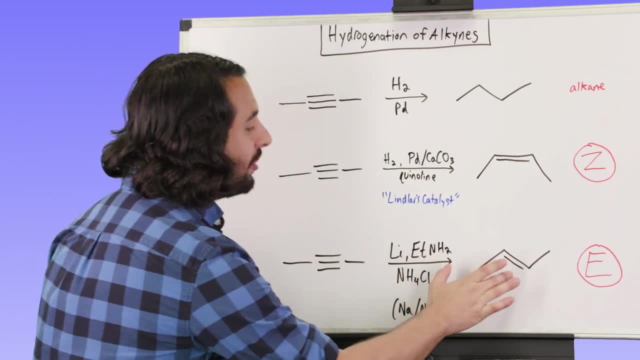 group level. It's going to take the alkyne. Okay, Okay, Okay, Okay, Okay, Okay Okay. It's going to go to the alkene, but it will specifically go to the e-alkene. So these are three things that we want to remember. 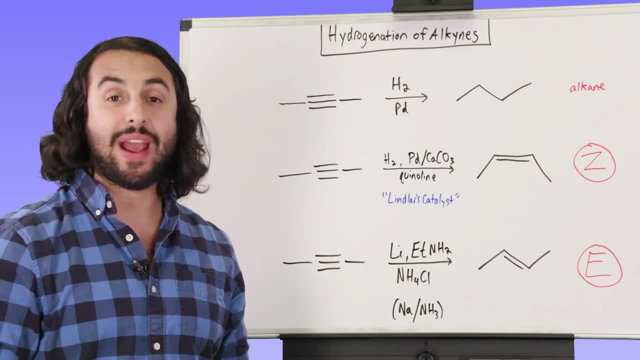 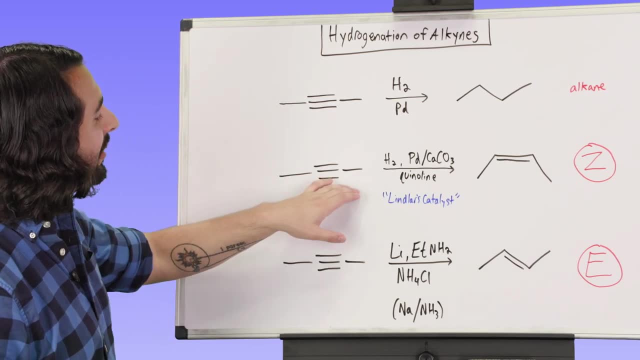 In terms of hydrogenation of alkynes, we have three ways that we can go. We can go all the way to the alkene with simple hydrogenation over palladium metal, or we can use Lindler's catalyst and go to the z-alkene, or we can use one of these two situations. 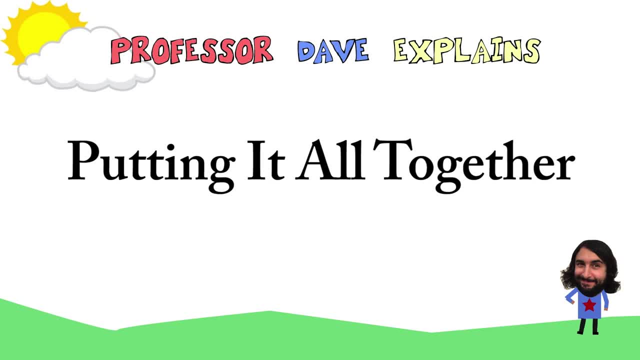 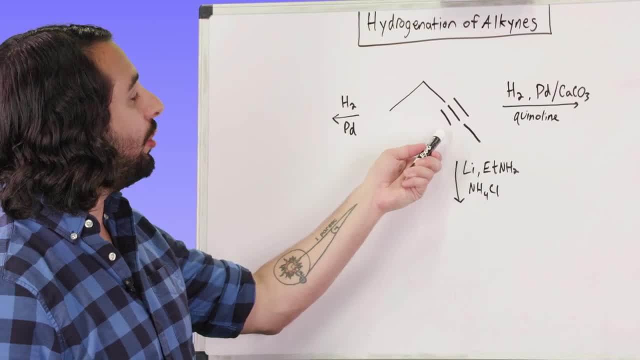 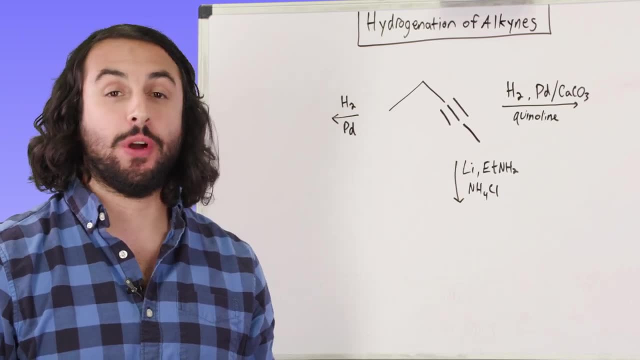 and go to the e-alkene. So let's put this into context. Let's say we're looking at this molecule, this alkyne, and we are going to attempt three different kinds of hydrogenation. Let's make sure that we understand what the product is going to be in each of these cases. 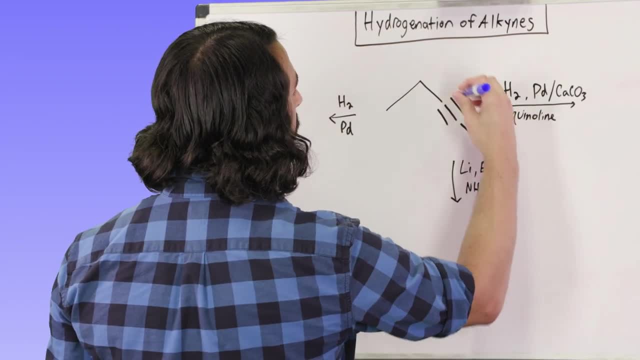 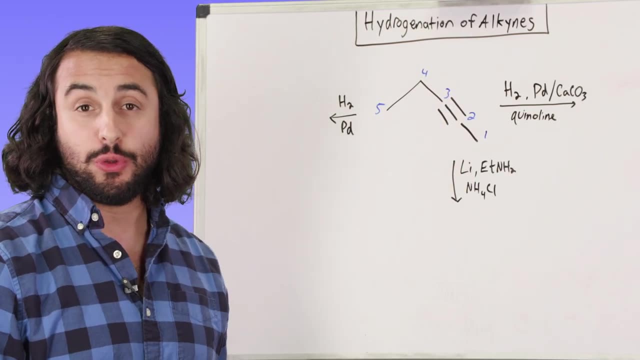 So we've got an alkyne. This is a one, two, three, four, five carbon alkyne Really quickly. A lot of times We're going to encounter some confusion when depicting alkynes. It does have to have this geometry and these are carbons, right there. 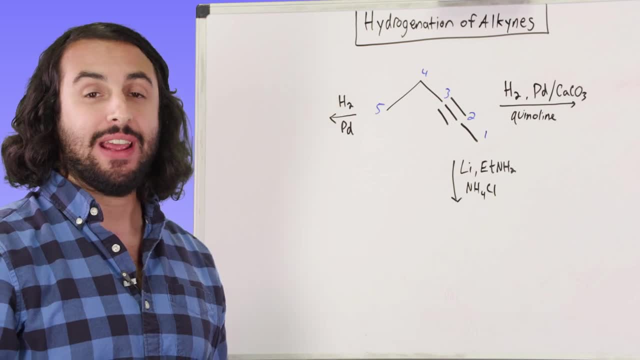 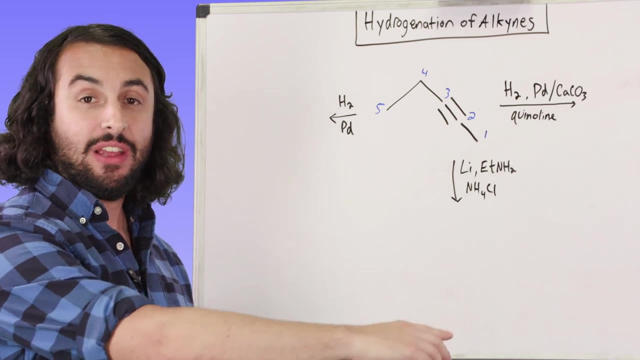 Remember that carbons participating in triple bonds are sp-hybridized and therefore exhibit linear geometry, So this is the right way to draw that right. We can't have alkynes in a zigzag fashion, because that doesn't depict the geometry accurately. 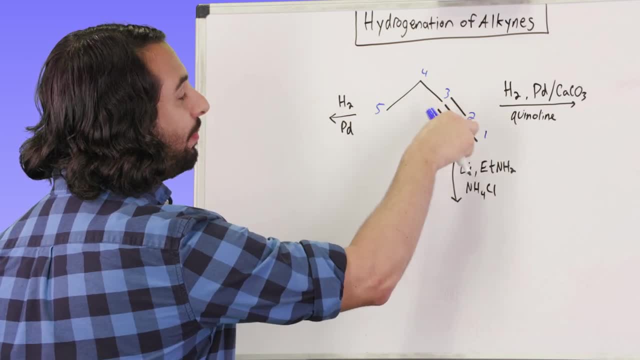 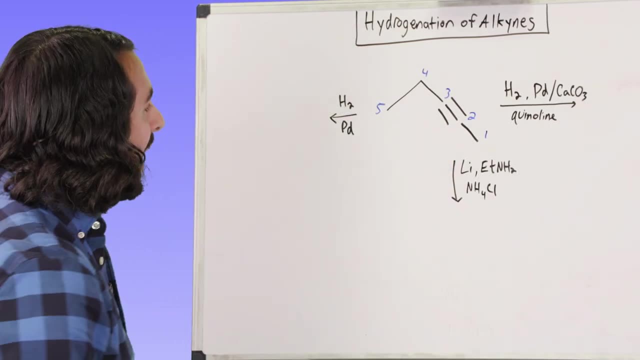 We do have a carbon here, and then two and three are triple bound, and then four and five. So this is a five carb. This is two carbons. One, pentane, would be the IUPAC name, and now let's say that we're going to do these. 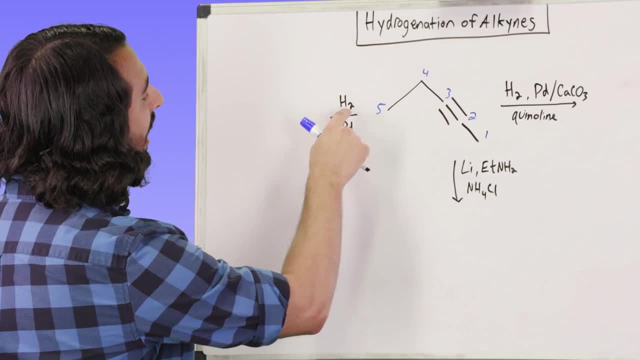 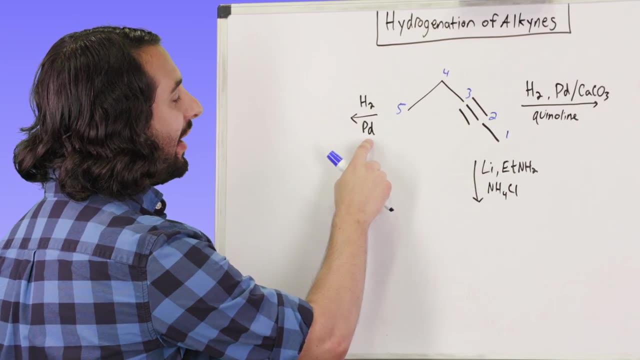 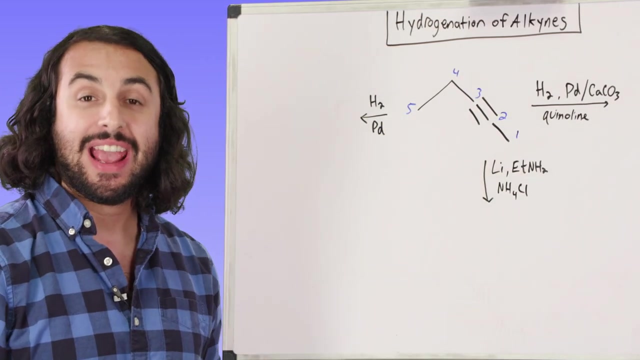 three different kinds of hydrogenation here. Let's say we do hydrogenation over palladium, and so what are we going to get? Well, we know that when we do this, we are not able to stop at the alkene right. This is going to hydrogenate, it's going to react with both of those pi bonds and we're 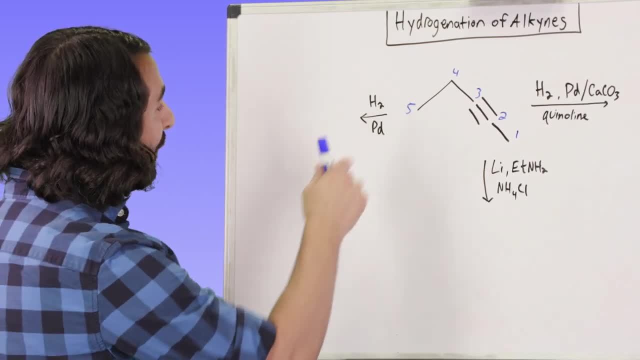 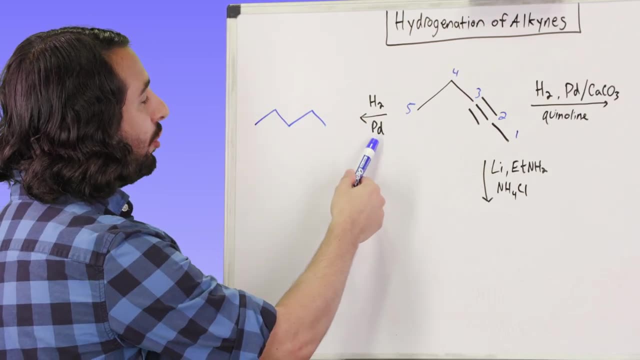 going to go all the way to the alkane. So we're going to get a five carbon alkane. We're going to get pentane Right there. So that's what's going to happen if we use those conditions for hydrogenation. 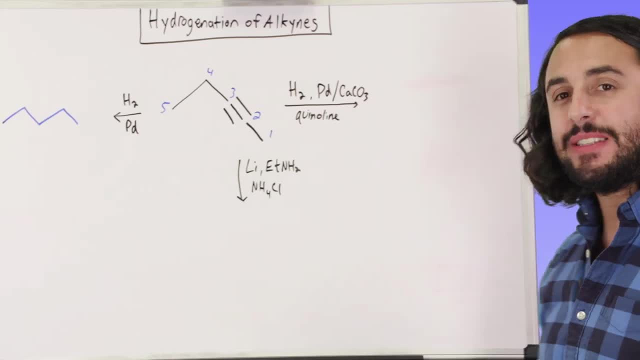 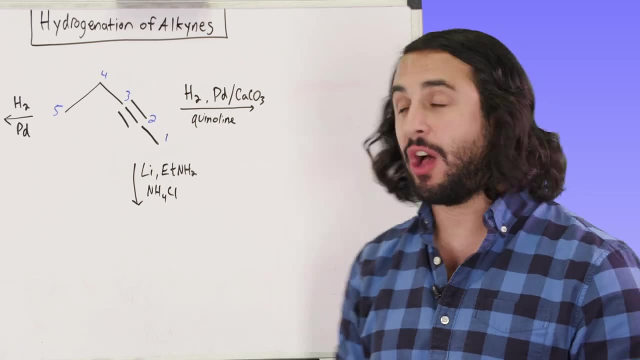 Now let's look over here. Now, what is this? We need to be able to look at conditions and, as best we can, sort of memorize what they do, so that on a test we know what to draw. and we should recognize that this is Lindler's. 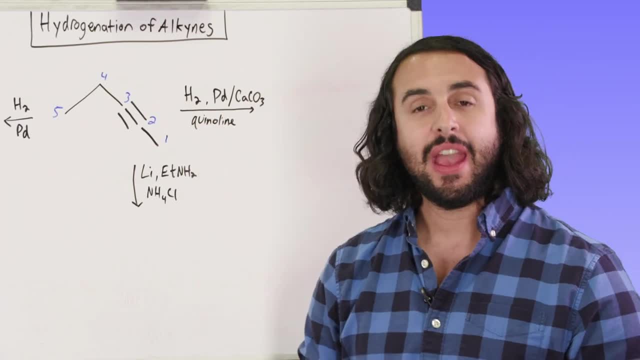 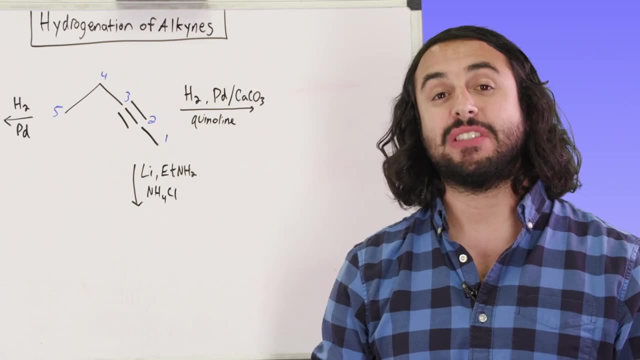 catalyst- Or, once again, we might just see Lindler right there- And what we want to associate in our minds is that Lindler's catalyst is always going to stop at the alkene, And it specifically will stop at the Z alkene. 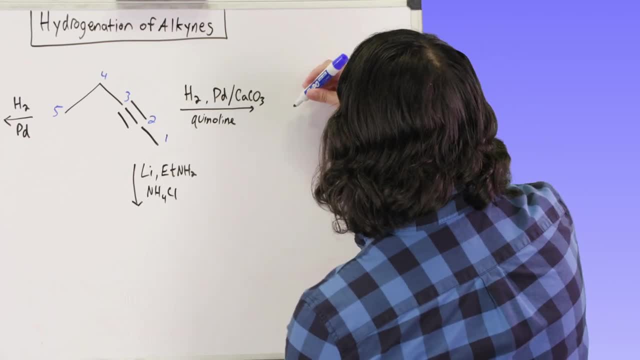 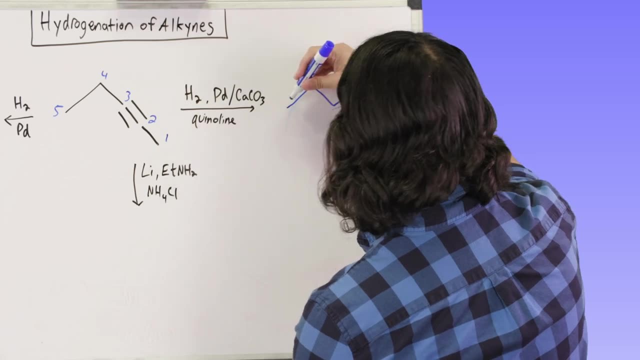 So we're going to get a five carbon alkene, right, So we're going to have a one, two, right. This is going to beand so one, two, three, right, It's going to connect these two, but they're going to be Z. 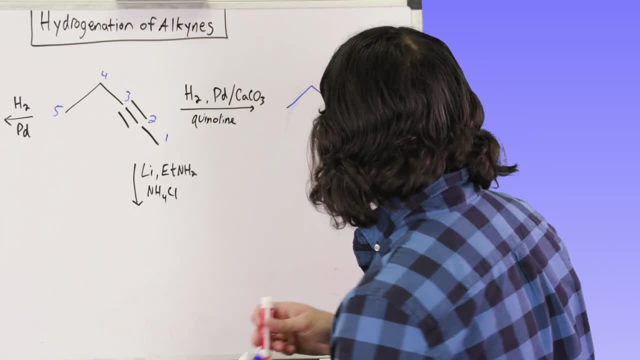 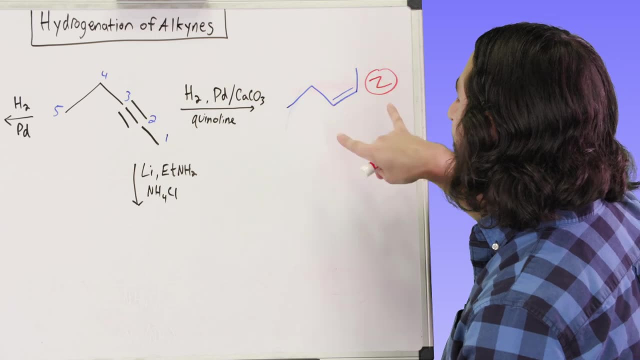 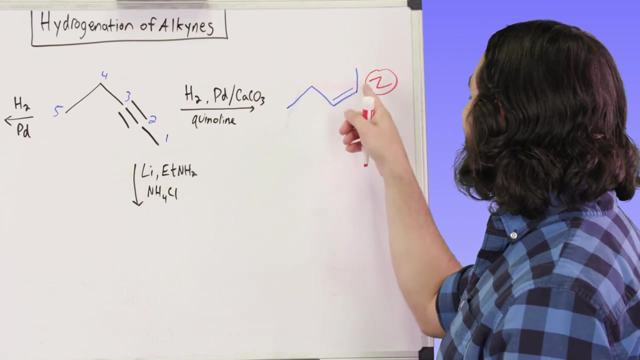 It's going to be a Z alkene, right? So this necessarily has to have this orientation, Right. So we need to have these alkyl groups projecting in the same direction, because Z-xam-xide, So one, two, three, four, five, that is a five carbon alkene. 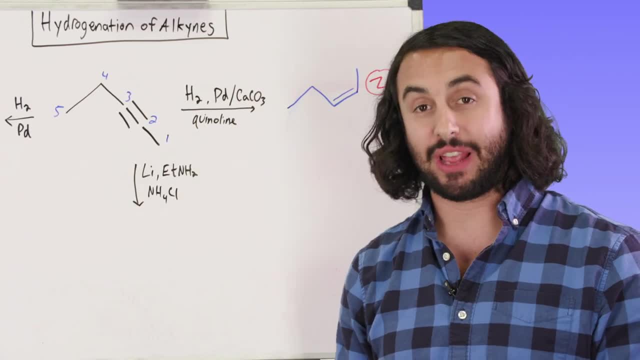 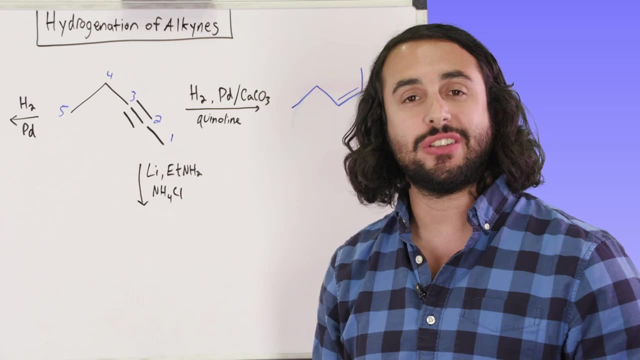 This is in the correct position, and we also have the correct stereochemistry at that location, And so we've got the Z alkene. that leaves our last situation. here We could have these conditions, or, once again, you may often see sodium and ammonia. 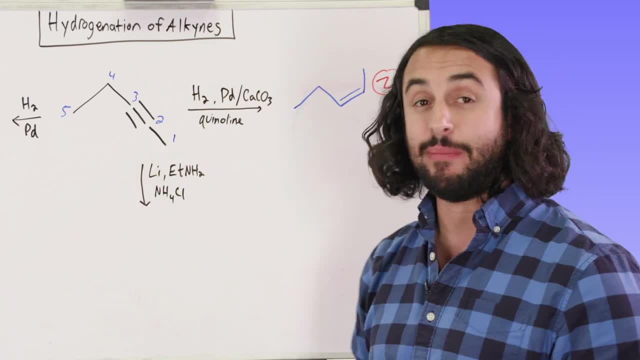 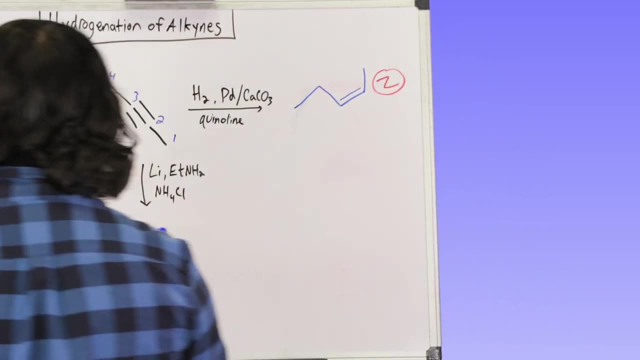 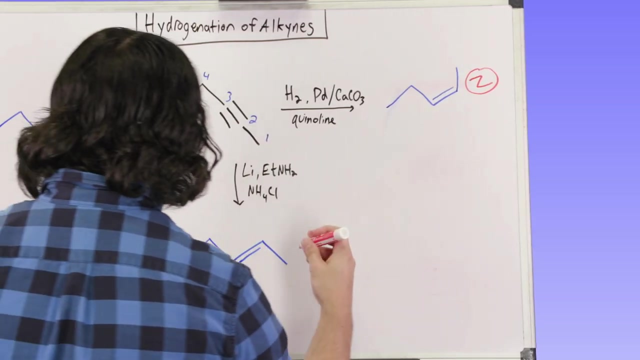 And so when you see something like that, again we're looking for this alkali metal there- lithium or sodium. That's what's going to be doing the chemistry, And we are going to get again the five carbon alkene, But now we are going to get the E alkene, right. 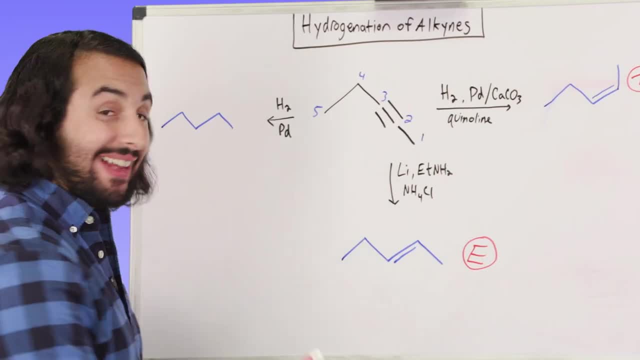 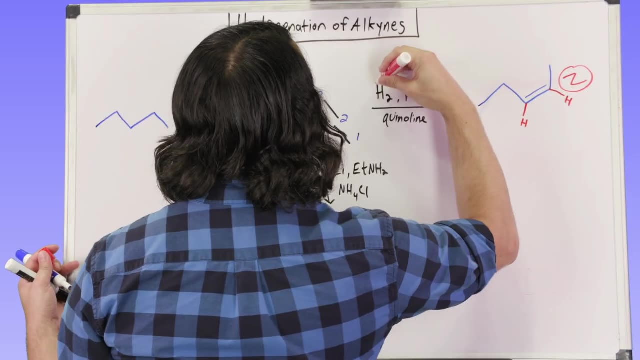 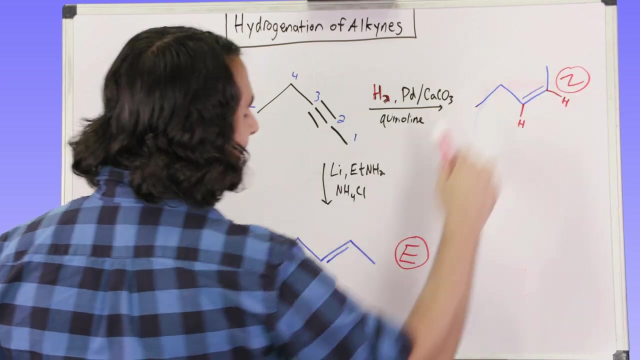 So the E alkene has the alkyl groups projecting in opposite directions. So whereas over here, right, these are the hydrogens, right there Those are the ones that got on there. So the hydrogens added to the same side we've got Z-xam-xide. 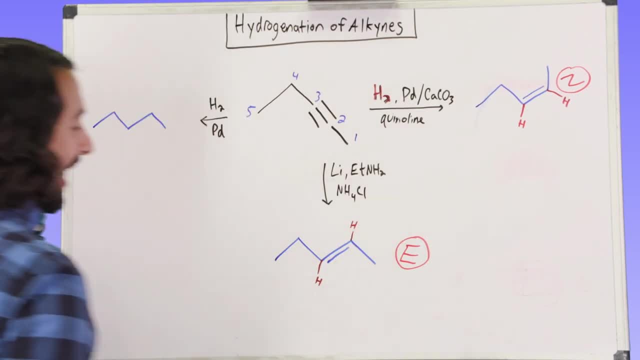 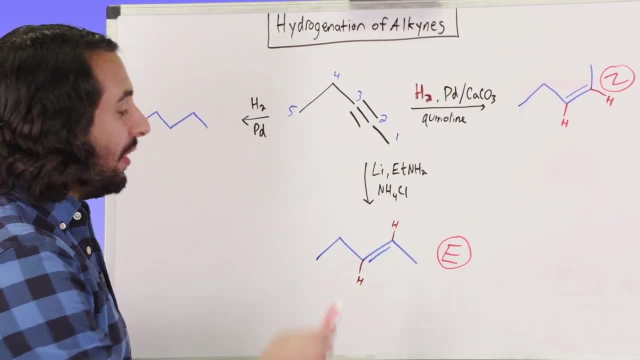 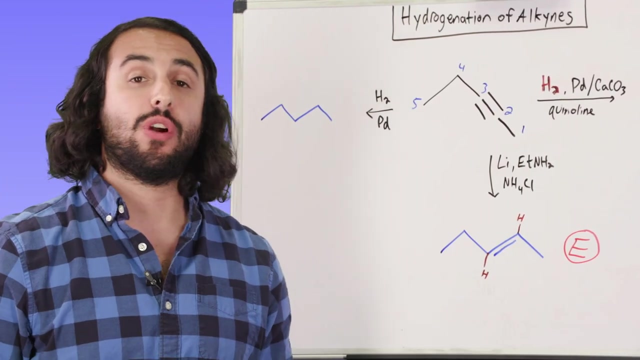 Over here we added these two opposite sides, okay, So we've got the alkane, we've got the Z alkene and we've got the E alkene, And hopefully that helps us understand these three different sets of conditions for hydrogenation.